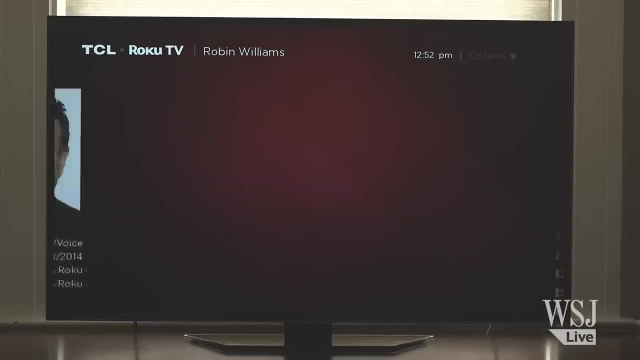 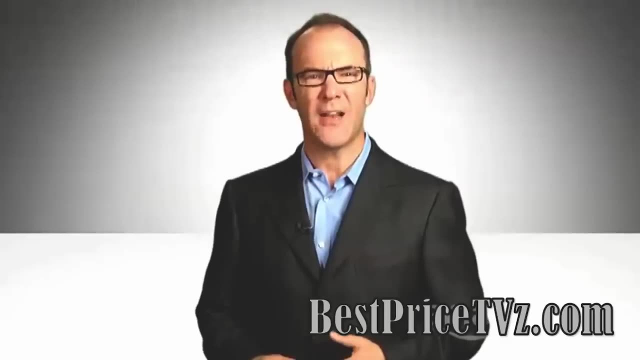 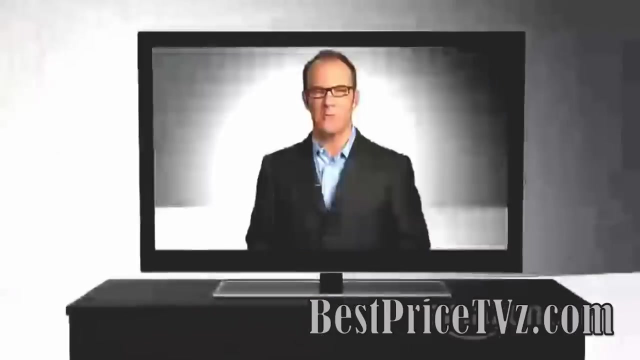 It's like Google for video: One place to find shows, movies or actors. What have you been watching? Admit it, you're tired of your TV just being your TV. It hangs out in your living room, It takes up space, It never cleans up after itself, It just shows TV. 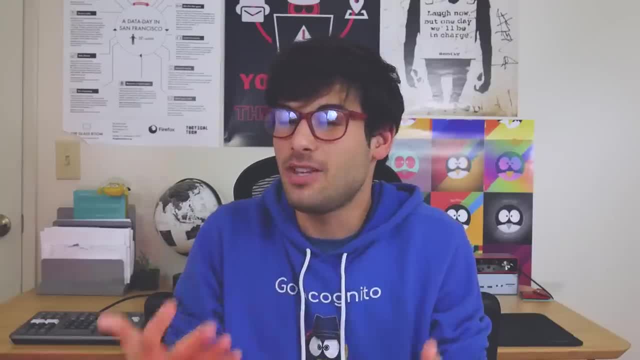 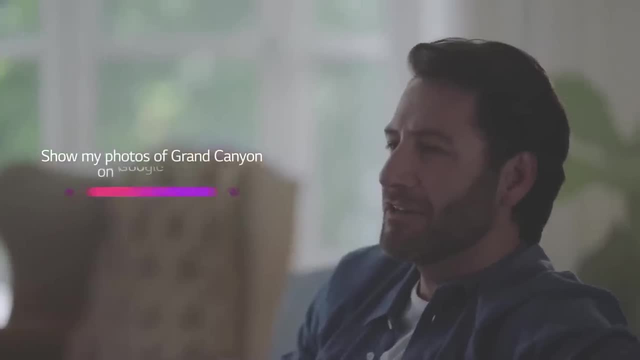 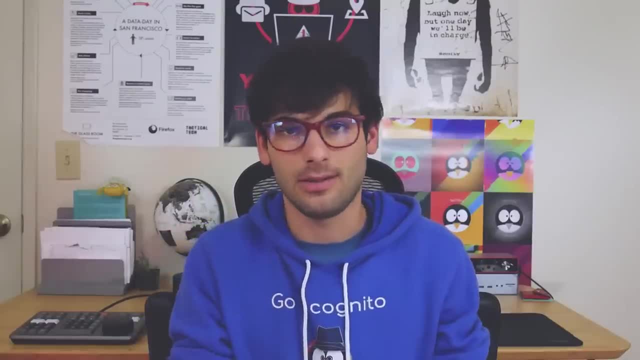 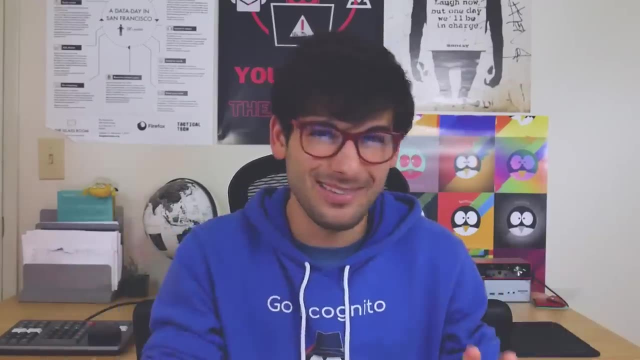 The idea that every device in your life needs to somehow do everything is ridiculous, since specificity is oftentimes a good thing and allows devices to excel where they need to. With TVs, the idea of them just being an amazing TV visually, with good support for other devices. 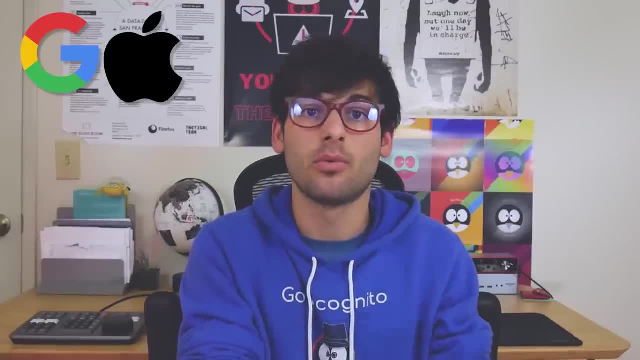 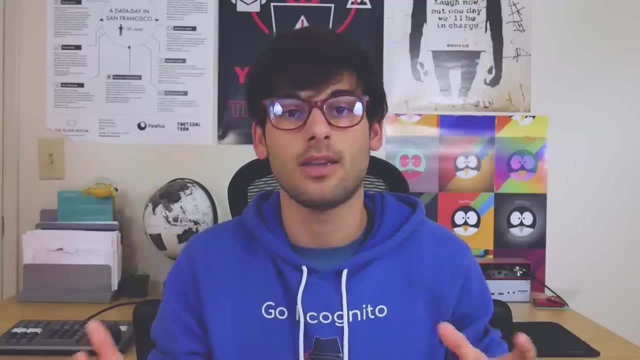 is just a clear win. Allow the companies like Google, Apple, Roku, Amazon, Sony and countless others to make specific devices with specific use cases. The idea that your TV will do everything is just a dream. You will still buy a Chromecast. 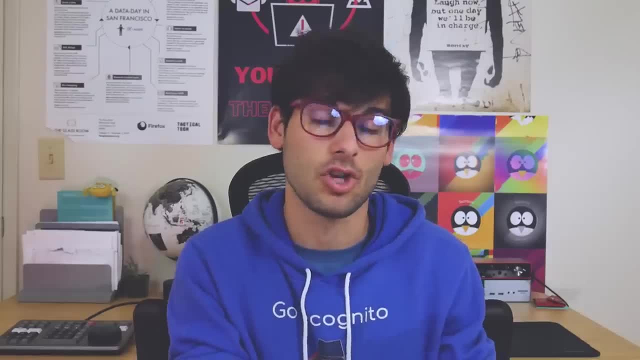 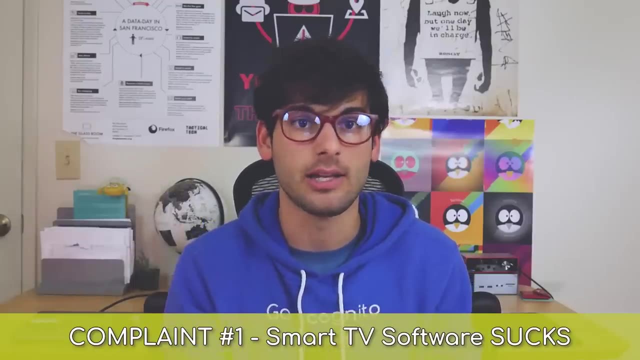 You'll still hook up a PlayStation to your TV, because those devices are actually good at what they do and improve your life. And that's complaint one. I genuinely think the software on these TVs just suck, And if I were to secretly replace my friend's TVs with dumb TVs, 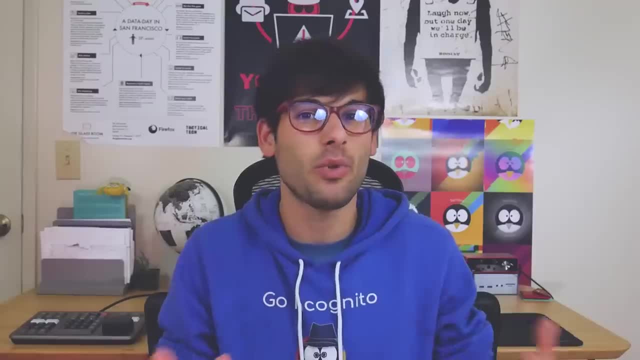 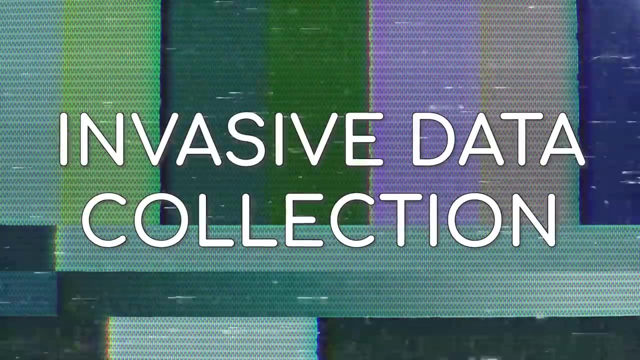 I feel like most of them wouldn't even be impacted much and some may not even realize because they literally just use their TV as a damn TV, not as some lockdown crappy home computer. Vizio was caught red-handed turning mountains of user data into cash by selling consumer. 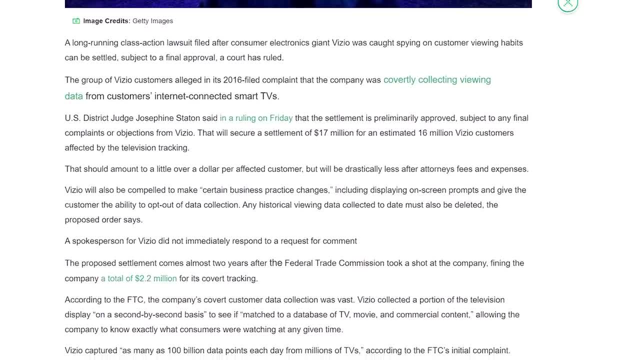 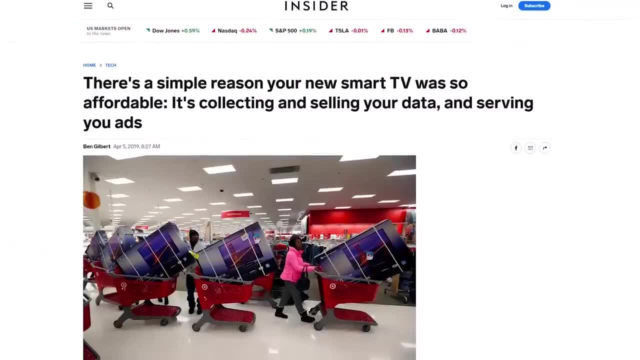 viewing history and other data to data aggregators, who were further targeted by trackers and advertisers- all, of course, without user consent or knowledge. A wonderful Business Insider article talks about the cutthroat TV data industry, where devices are undersold due to the amount of money being made on user data. 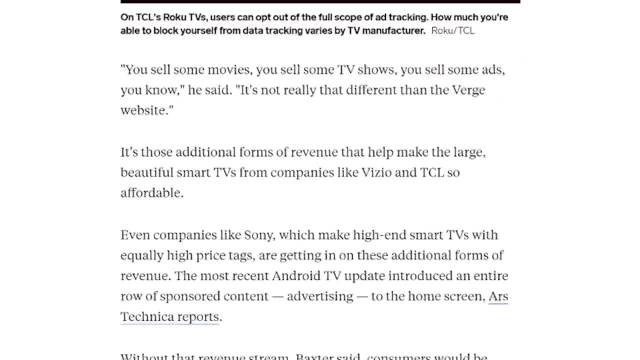 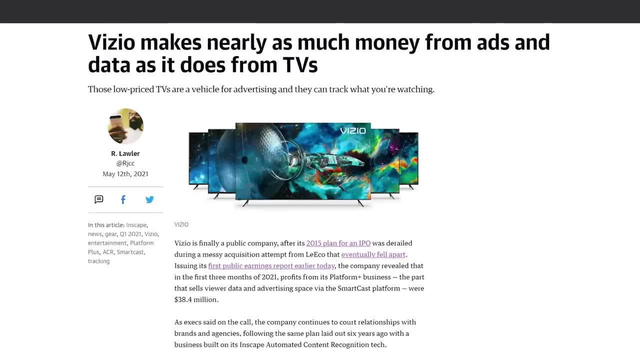 including things like their approximate location. the ads watched, the kinds of shows and more. Vizio, specifically, doesn't even need to make money from every TV they sell and are able to take a hit because of how lucrative this industry is. As a matter of fact, they recently made $48. 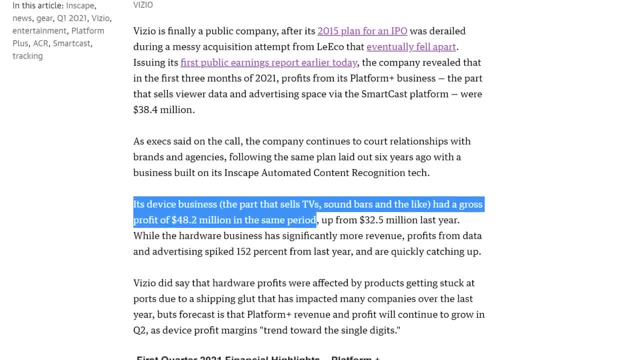 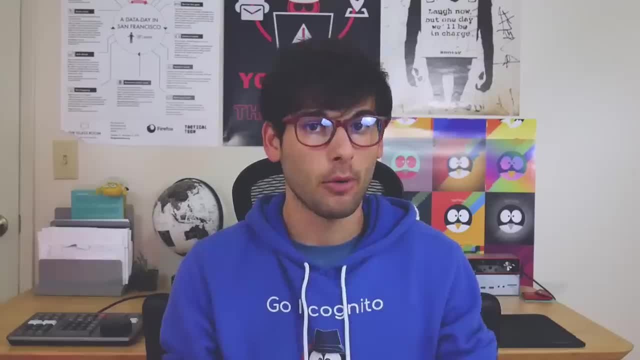 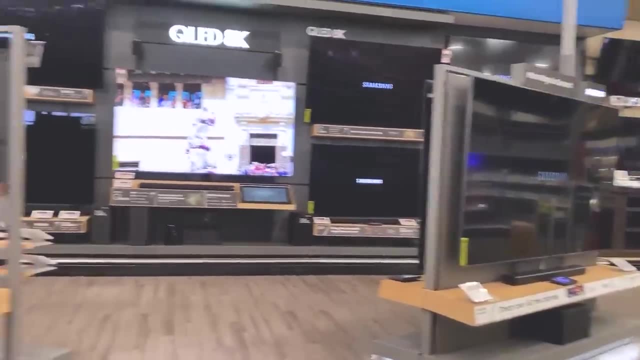 million on hardware in one quarter and in the same period, made $38 million, meaning they've already made almost the same amount of money between data and hardware. Most other TV manufacturers are likely experiencing the same thing, which explains the inability to even find a damn non-smart TV. 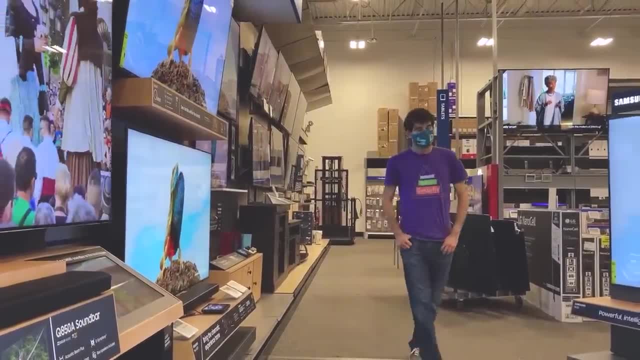 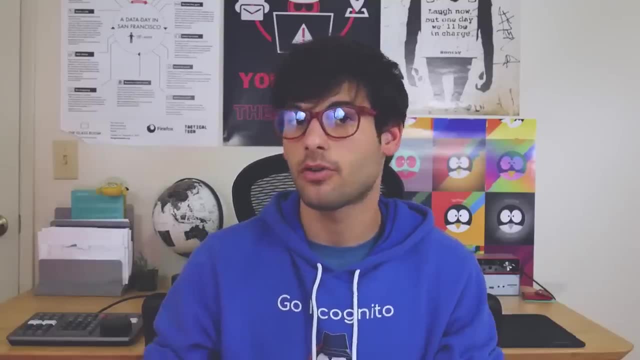 It's just so hard, It's just more lucrative to make smart TVs than to not. This isn't done with your best interest in mind. of course, Some of you may be completely okay with paying less for a TV in return for some data. 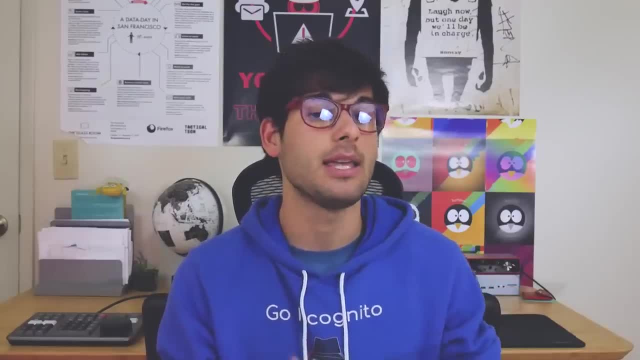 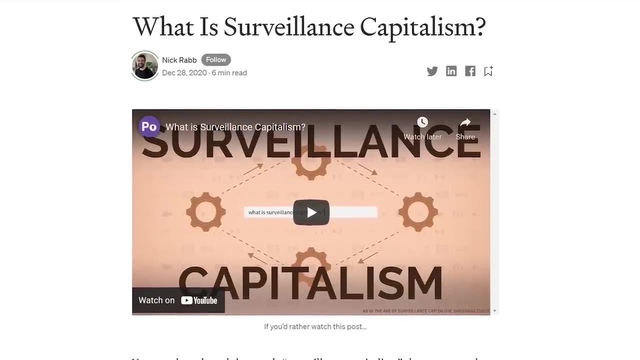 collection, but I would challenge you to think differently about how that is your data, and you shouldn't sell out your personal information. Surveillance capitalism is a very real thing, and this is just one of many ways it's revealing itself in our society, along with the countless other IoT devices continuing the same direction. 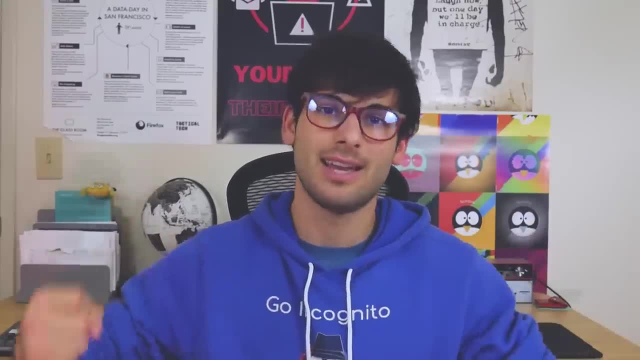 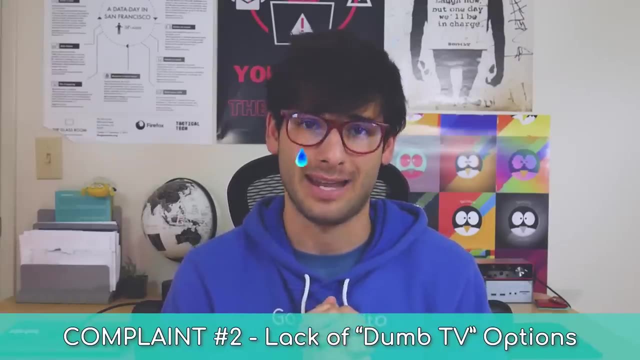 I would gladly pay more for a TV I can confidently trust is respecting me and my data, but this option is becoming almost impossible to find nowadays, which is just so sad. And finally, we can't talk about data without talking about privacy and security. 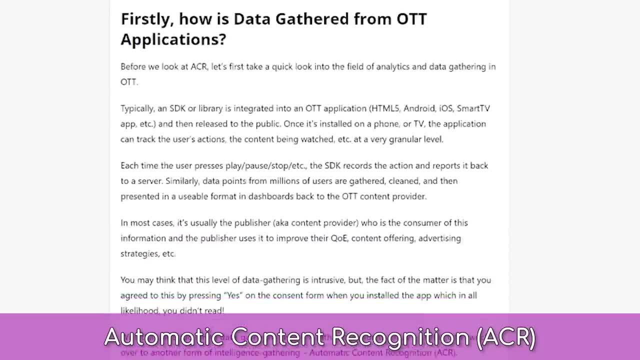 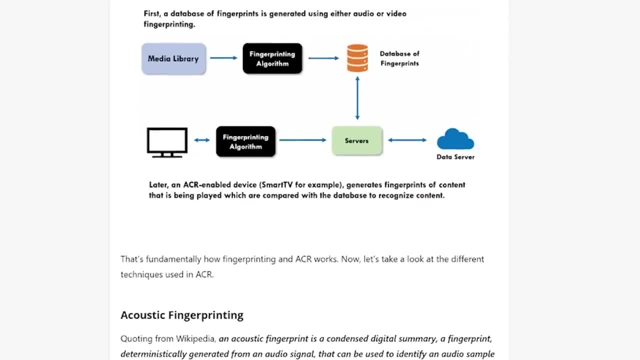 ACR is called automatic content recognition, and most modern TVs implement some form of this technology. What it is is like having an ad executive watching you watch your TV, analyzing everything you're doing, so they can capture and sell this information to the highest bidder. 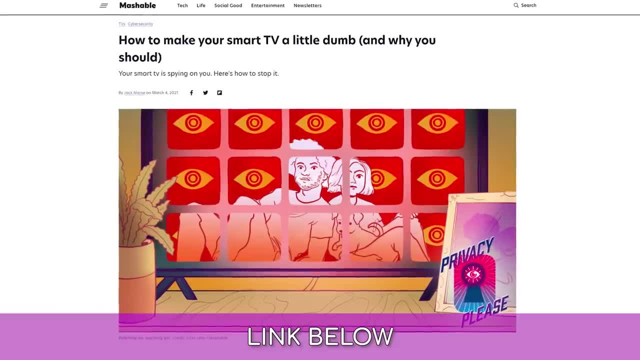 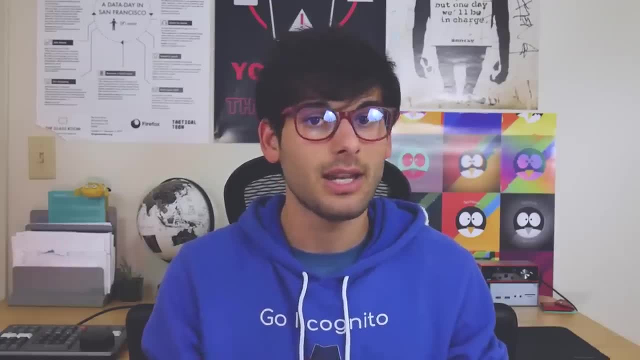 This is clearly a privacy violation, and this wonderful, Mashable article talks about how to turn off ACR in most situations. Every single thing you do on your TV, you should assume, is being sold and collected without your explicit knowledge and consent, which is just really fun. 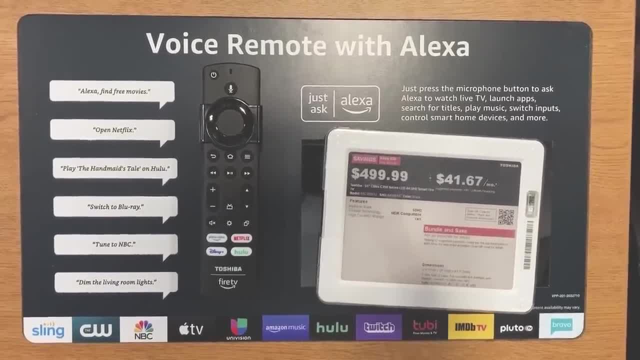 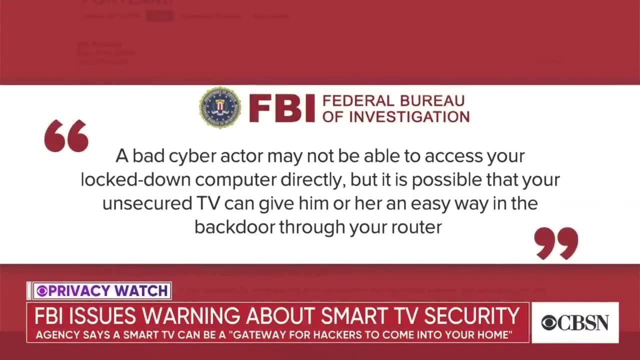 Aside from this, many TVs come with microphones and cameras, which pose their own risks. Last week, the FBI posted about the risks of having a smart TV on its website. The agency says the devices can be gateways for hackers to access your home. 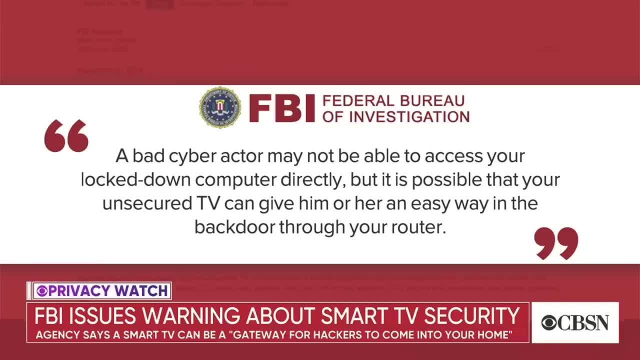 and other devices because they are connected to the internet. That means hackers can take control of your unsecured TV and play with its settings and, in some cases, take control of your TV's camera. I've seen it happen before and I'm sure it's true, But it's also a risk.